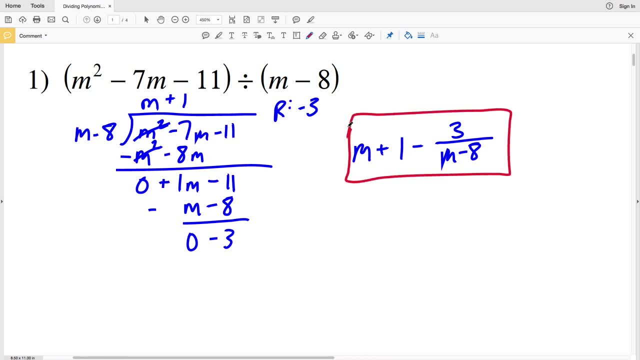 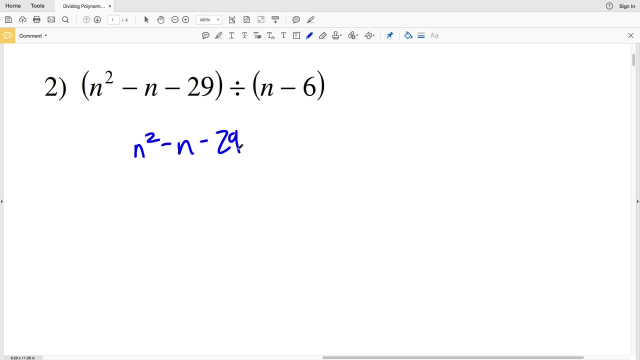 our solution is m plus 1 minus 3.. 3 over m minus 8.. On to number 2,. we have n squared minus n minus 29, and we're dividing that by n minus 6.. So again we're looking at n. and how many times does n go into n? 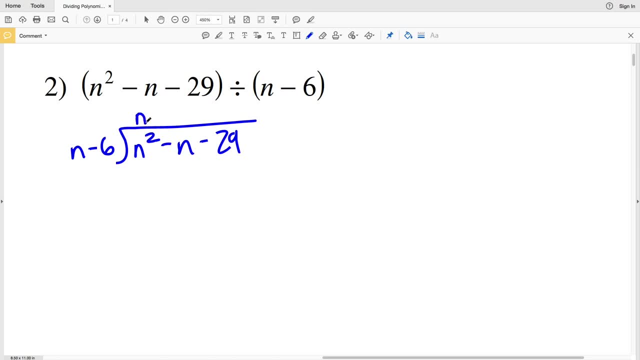 squared n goes into n squared n times. So we're going to take this n and multiply it by n minus 6.. That'll give us n squared minus 6n And we're subtracting this. So we're going to doing that. So n squared minus n minus n squared minus 6n- n squared- will cancel out Negative. 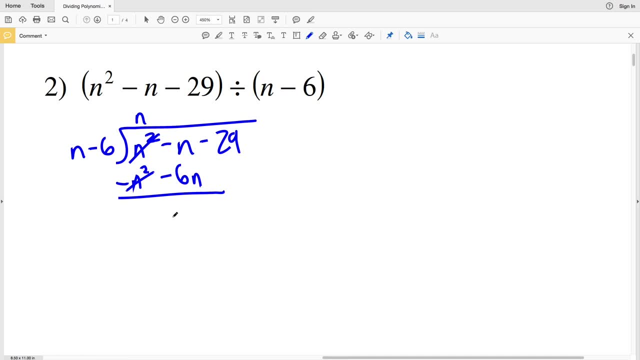 n minus negative 6n is going to be a positive 5n, and we're still subtracting 29.. Now we have to see how many times n goes into 5n, And that's 5 times And it's a positive 5.. 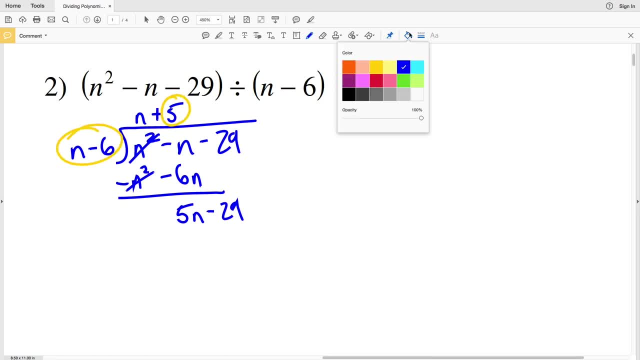 So now we're going to take that positive 5 and multiply it by n minus 6 and subtract that quantity. So 5 times n minus 6 is 5n minus 30. And we're subtracting that, So 5n will cancel. 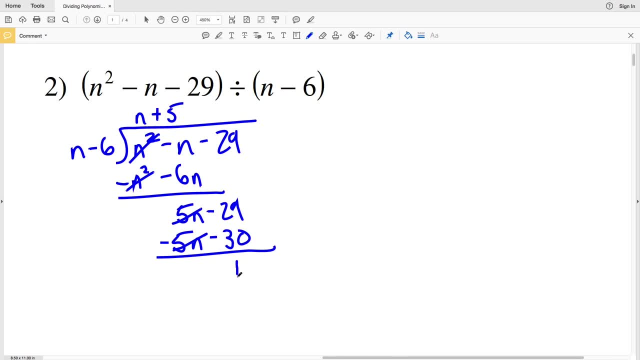 out, And negative 29 minus negative 30 is a positive 1.. So this time our remainder- I'll say r- is 1.. So our answer is n plus 5 plus, since our remainder is positive, 1 over n minus 6.. n plus 5 plus our remainder of 1 over n minus 6.. 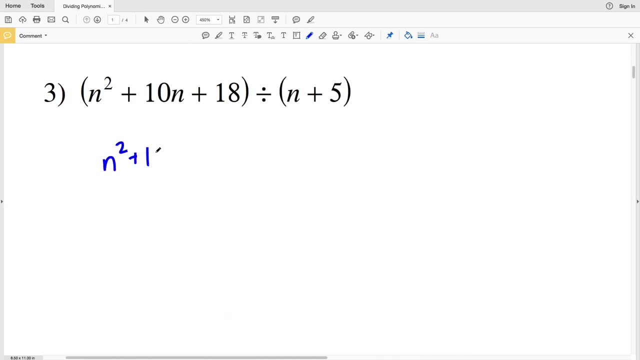 And number 3, n squared plus 10n plus 18 divided by n plus 5.. Looking at the n at the start, n goes into n squared n times n times n is n squared, Then we're going to take this n. 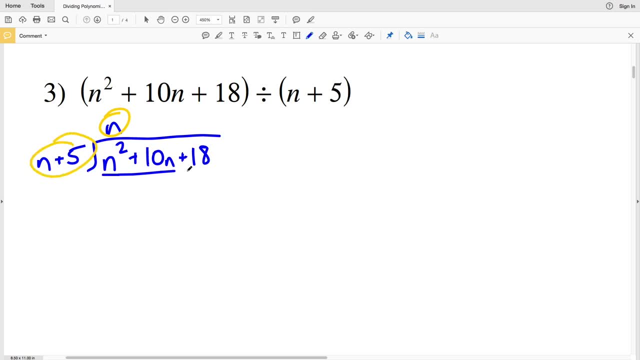 and multiply it by n plus 5 and subtract that from our polynomial, So it'll be n squared plus 5n and that's subtracted, n squared will cancel out 10n minus 5n is a positive 5n, And we're still adding that. 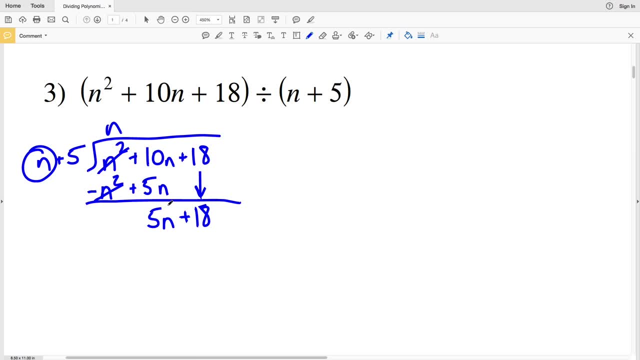 18.. Now, looking back at n, that goes into 5n, a positive 5 times. So 5 times n plus 5 is going to be 5n plus 25.. And we're subtracting that, So 5n will cancel out 18 minus 25 is. 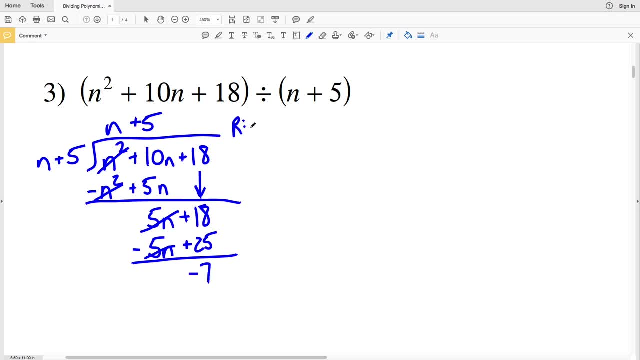 a negative 7.. So our remainder is negative 7.. So our remainder is negative, 7.. So our solution: n plus 5, minus, since our remainder is negative, 7 over n plus 5.. So again, our answer is n plus 5 with a remainder of 7.. So that's n plus 5 minus 7, over what? 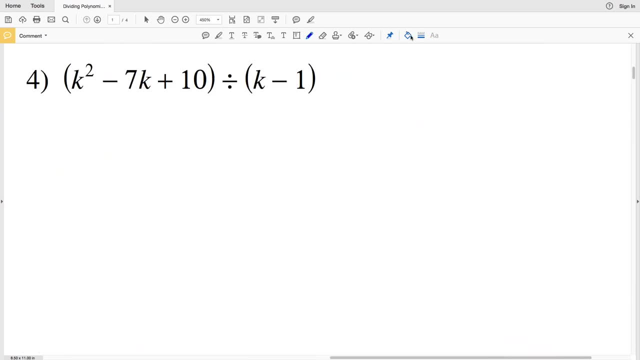 we divided by n plus 5.. And number 4, we're dividing by n plus 5.. So that's n plus 5 minus 7 over n plus 5.. We're adding k squared minus 7k plus 10 by k minus 1.. Starting with the k, k goes into: 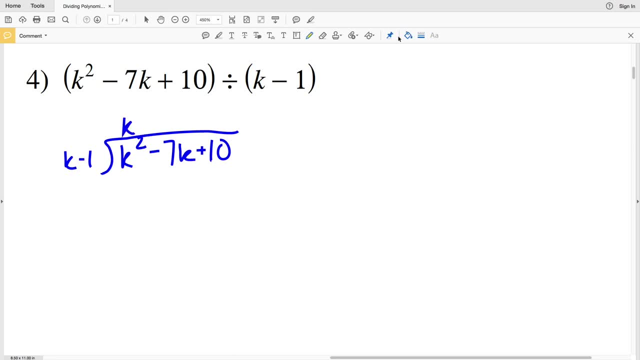 k squared k times. So now we're going to multiply this k by k minus 1.. That will give us k squared minus 1k And we're subtracting that, So k squared will cancel out Negative 7k, minus a negative 1k, will be negative 6k, And we're still adding 10.. 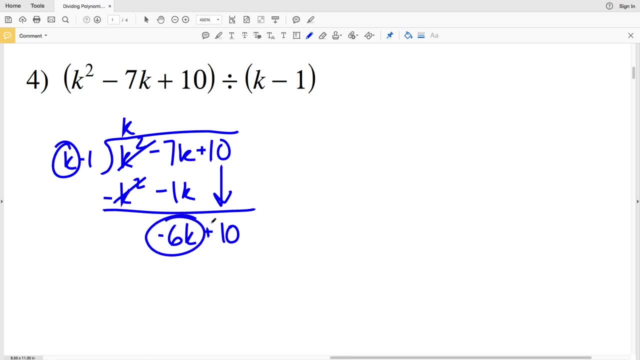 Now we're going to see how many times k goes into negative 6k And that's negative 6 times. or we could just say subtracting 6 from k. So now we're going to take that negative 6 and multiply that to k minus 1.. That'll be negative 6k plus a positive 6.. And when we're 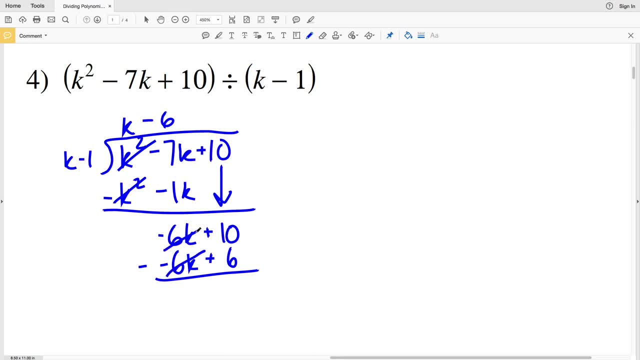 subtracting this, our 6k's will cancel out, since negative 6k plus 6k is 0.. And then we're going to add: 10 minus 6 is 4.. So we have k minus 6 with a remainder of 4.. Therefore, 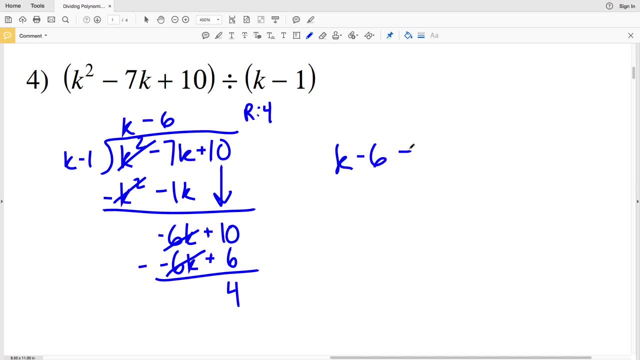 our final solution is going to be k minus 6 plus 4 over k minus 1.. k minus 6 plus our remainder of 4 over k minus 1.. And number 5, starting with n, n, goes into n squared n times. So k minus 6 is 0.. And then we're. 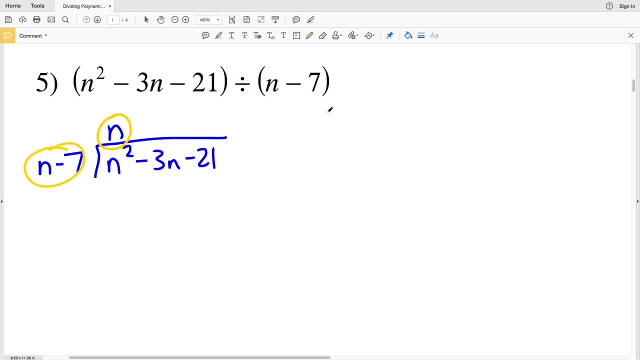 going to subtract that n times. So now we're going to multiply that n by n minus 7 and subtract that n times. n minus 7 is n squared minus 7n, And when we subtract that, our n squareds will cancel out Negative 3n minus a negative 7n is a positive 4n And we're subtracting that 21.. 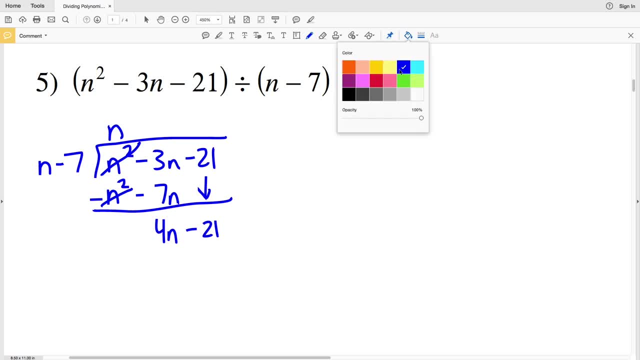 Now, how many times does n go into 4n? n goes into 4n four times, And that's a positive 4.. Now we're going to take that 4 and multiply it to n minus 7.. 4 times n minus 7 will be 4n minus 28.. 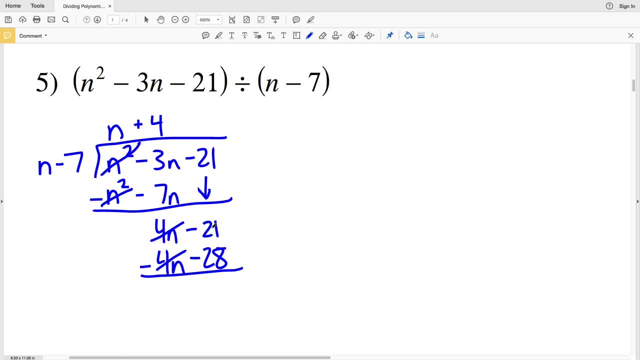 And we're subtracting that. So our 4n will cancel out Negative. 21 minus a negative, 28 is a positive 7. So our remainder is a positive 7. And you can see that our answer is n plus 4 with a remainder. 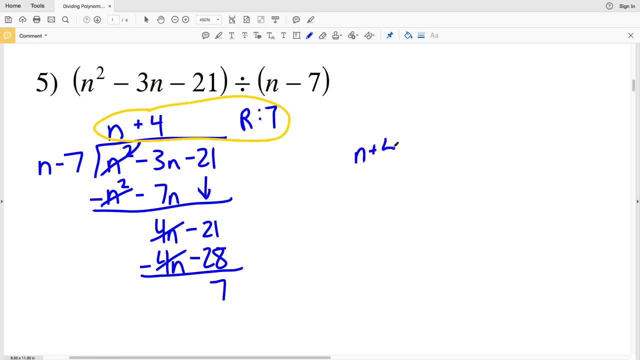 of 7.. So we're going to write n plus 4 plus 7. And we're going to subtract that 21 minus a negative 7.. Our remainder value over n minus 7, since that's what we divided by n plus 4 plus 7 divided. 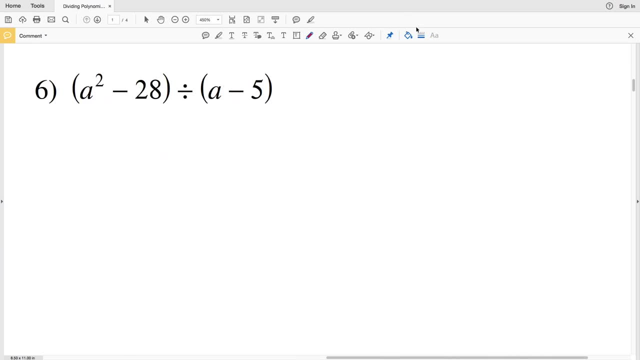 by n minus 7.. And lastly, in this video I'll go over number 6.. In number 6, we have a squared minus 28.. However, we're missing an a to the 1 or a value, So we're going to write a squared. 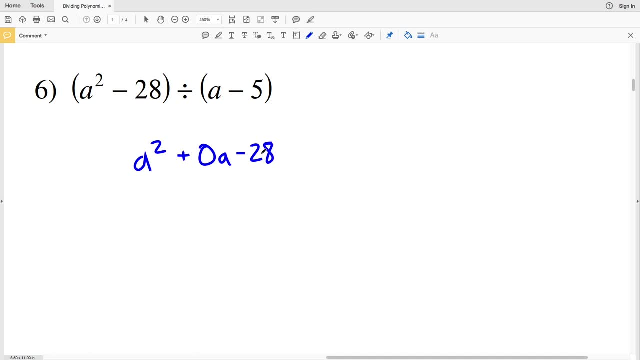 plus 0a minus 28.. Since a squared plus 0a minus 28 is the same as a squared minus 28,. since 0 times any number is 0. But we need that placeholder in there so we can divide, And we're dividing by a minus 5.. 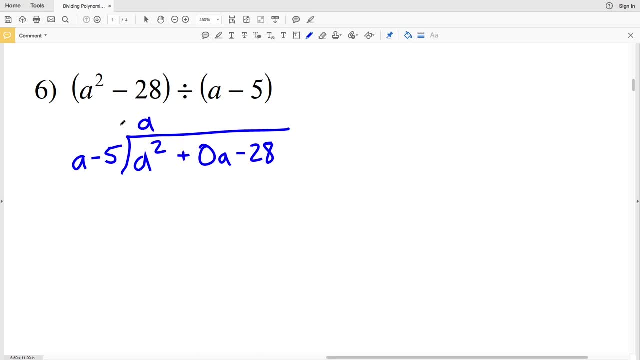 So a goes into a squared a times And then we multiply a times. a minus 5 is a squared minus 5a. Now you can see why I put the placeholder in. a squared will cancel out 0a minus negative 5a is a positive 5a And we're still subtracting.